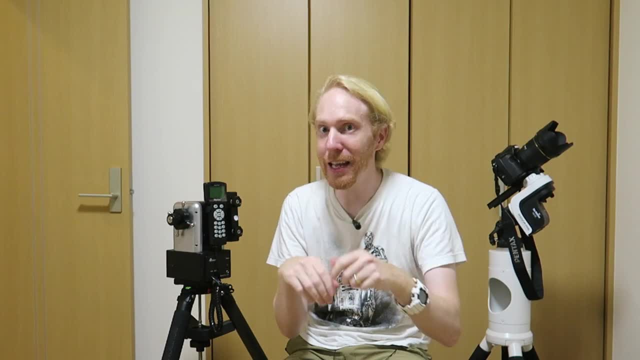 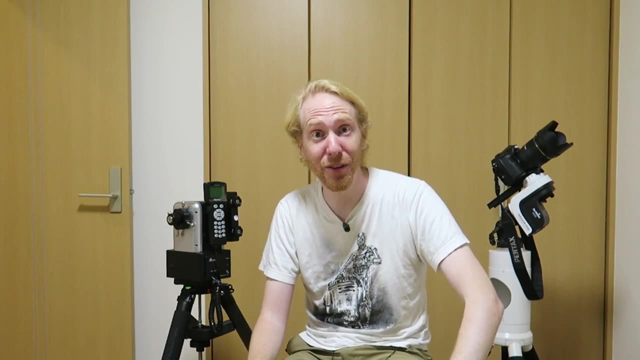 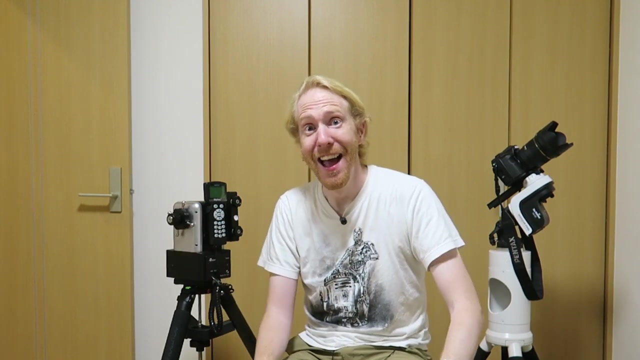 recently in Tokyo, and so I'm getting slightly- only slightly- desperate. And with that I've, you know, I've remembered that you can actually download raw files, raw fits, files from the Hubble telescope archive- It's all free and available- and process them, and so it's a lot of fun to do so. 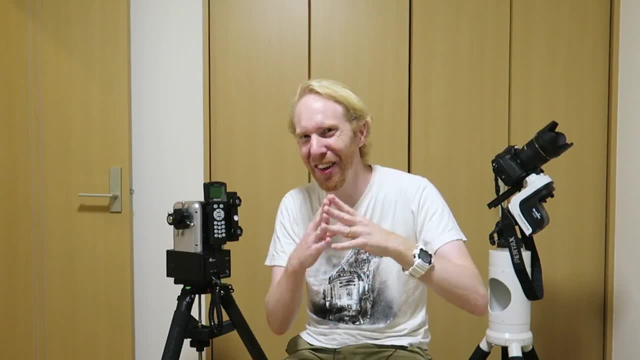 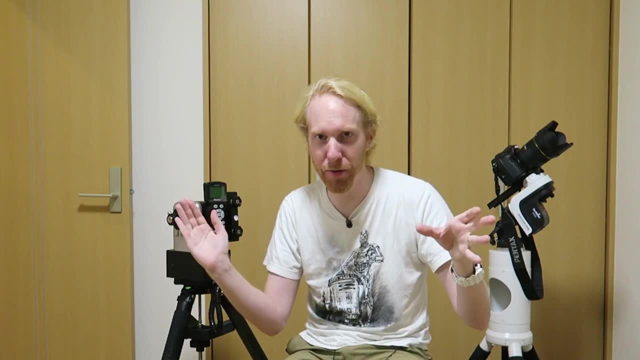 And in this video I want to go through how to do that, because it's not quite immediate: how to find all of those images and also the. the Hubble telescope has like millions of different filters, and so which filters should we use, in what situation? how to map them, something that makes 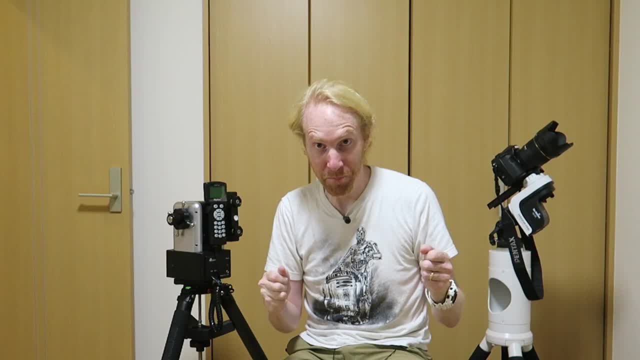 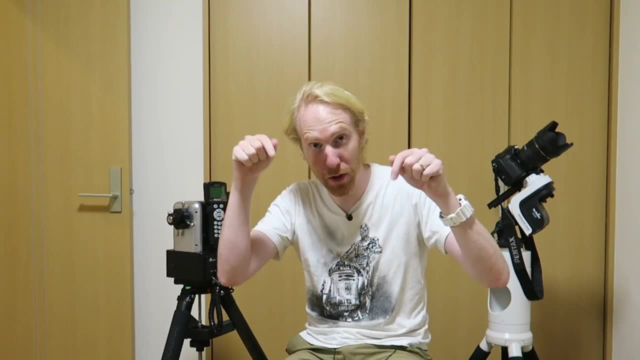 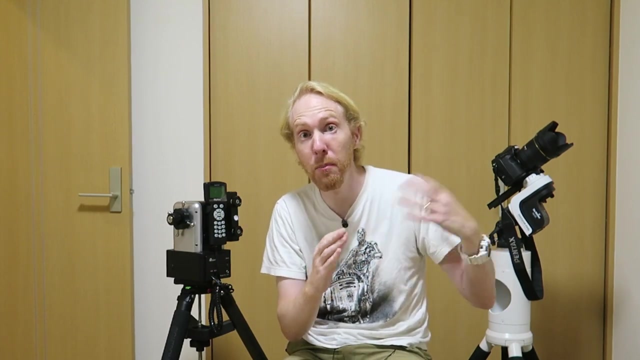 sense, It's actually really difficult to find out. So the reason I did that is I saw some other YouTubers, like Helena from Helena Astro, who's awesome, by the way. you can check her channel. I put a link in the description down below. but basically using remote telescopes that you can buy time from. 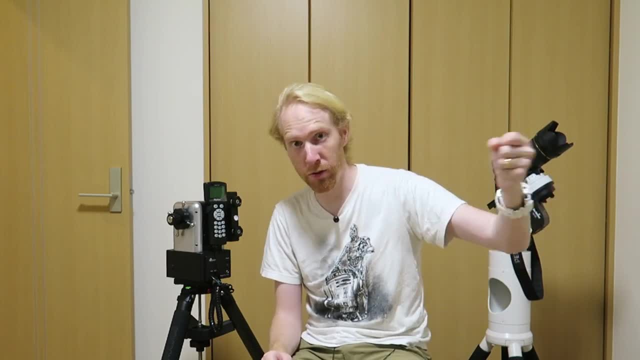 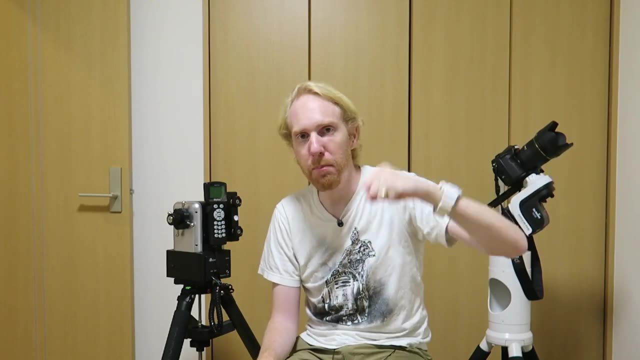 to take an image, except that you're not really controlling the telescope. you're just basically telling the people there, whatever, that you want an image of this with this exposure time, blah, blah, blah, and then you get back raw data that you can process. And here we're just going to get data. 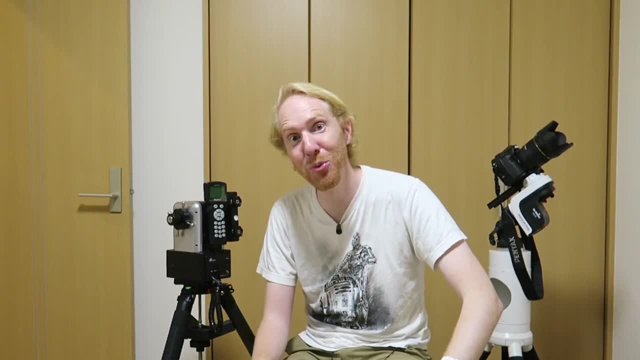 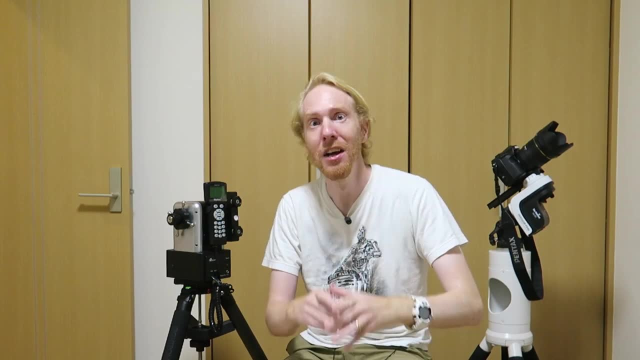 from the Hubble telescope. We're going to process it And we're going to compare it to whatever the big brains at NASA or whoever does the processing- I have no idea who does the processing of those images actually did, So let's do that. 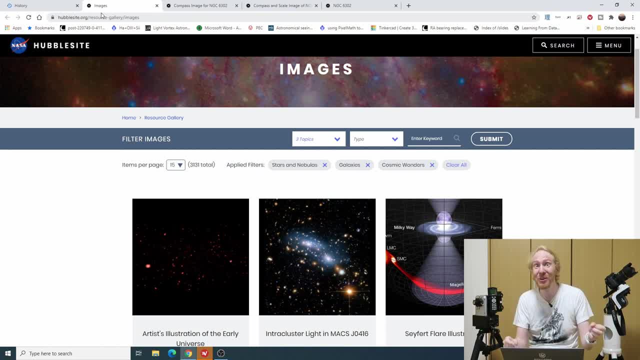 And so what I like to do to first start with is to go to a website called hubblesiteorg, and then you can- I'll put the link in the description down below- but in the resource gallery you have all sorts of images, and then you can filter those images. you know: stars, nebulae, galaxy, whatever. 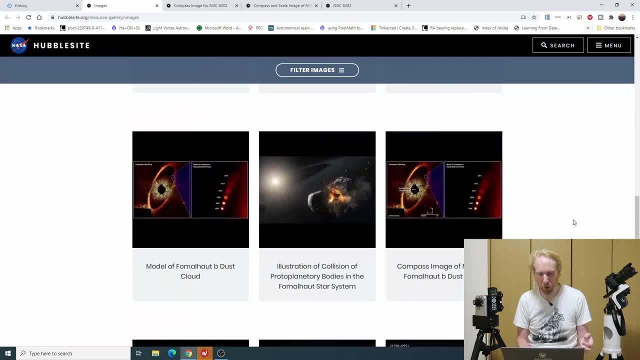 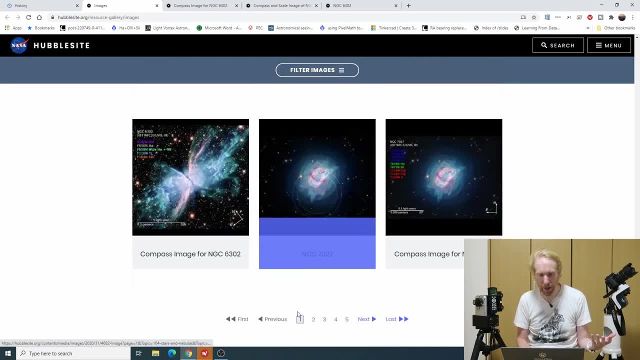 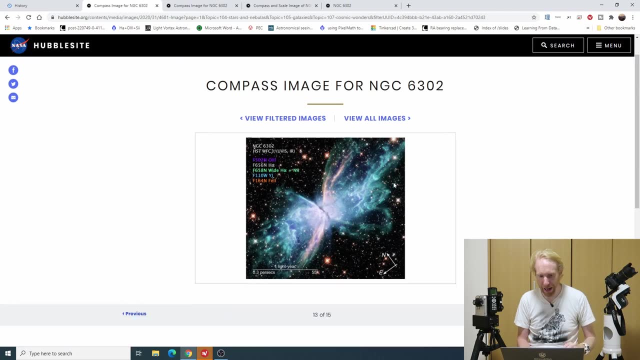 it's observations, all that kind of stuff, and it will show you a lot of you know images that come from that and I like to select. you know images that are of nebulae and like this one. this one is really nice because we have the image itself and we also know how it was processed. you can see. 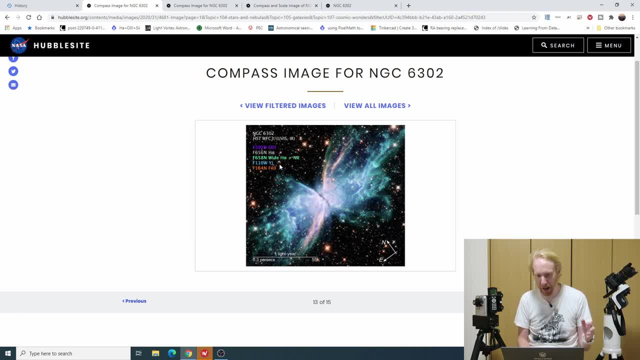 it has, like oxygen, 3, hydrogen alpha, hydrogen alpha and n2 and then whatever yj and fel are, you know things, and the numbers you see on the left hand side, like this f502n or f656n, f658n, you might remember, you might actually recognize the 656, 658, 60502 as being kind of like band, I mean wavelength. 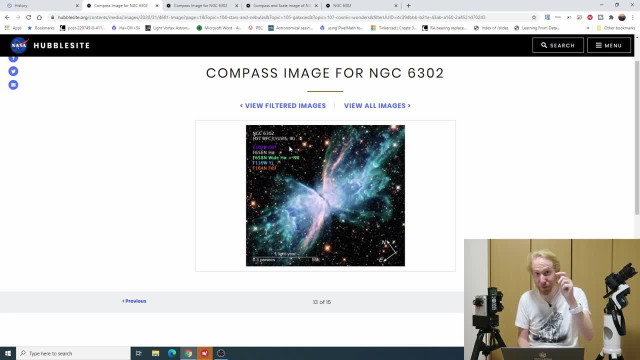 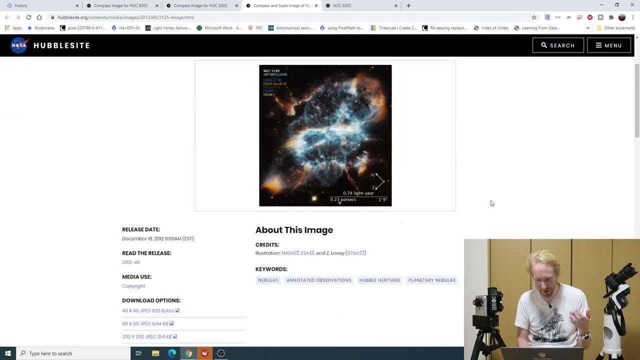 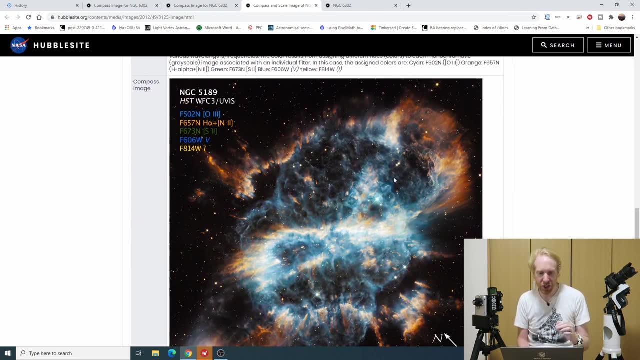 and it pretty much is the case, and this gives you the actual names of the filters used by the Hubble telescope. and one of my favorite images that I like to use is the one that I'm going to, that I see on here is: is this one of ngc 5189? and we can see this image has been taken with five. 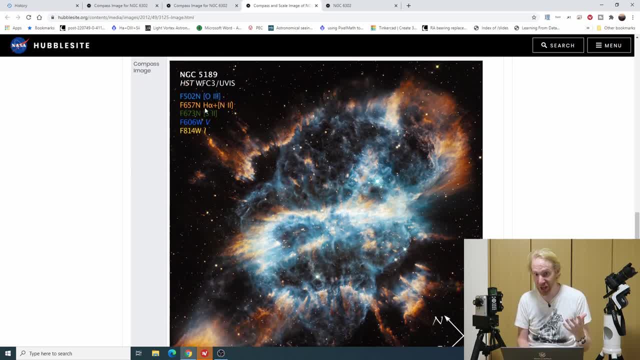 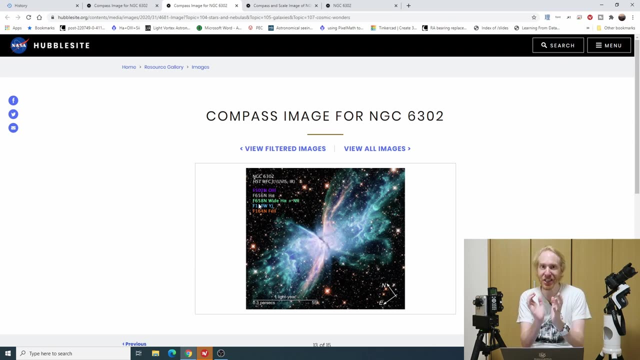 filters. one is oxygen 3 was, one is h alpha plus a bit of n2 and the other one is s2 and you can see it's 673 and you have like 656, 657, 658, like some are like h alpha, like the first one is h alpha. 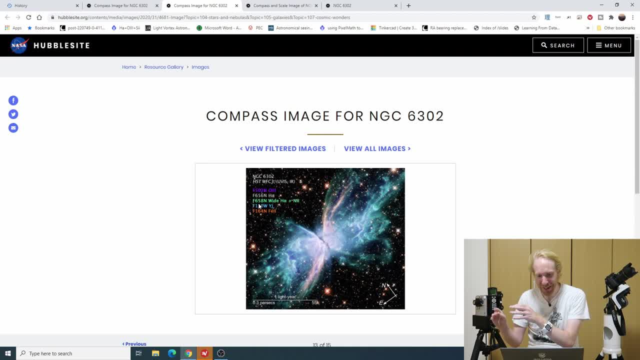 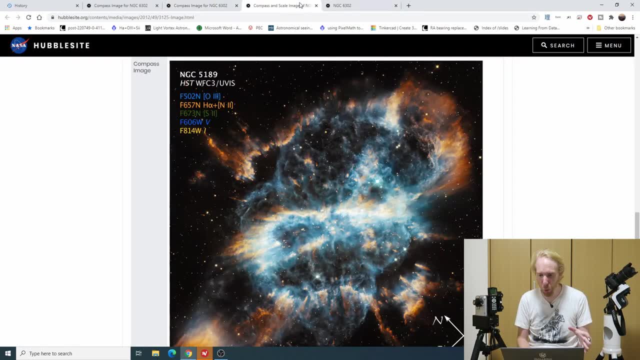 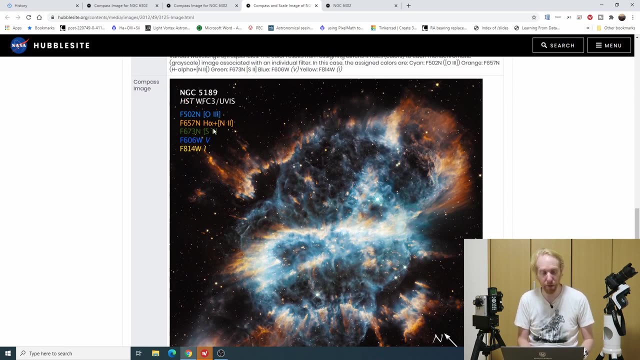 2. the third one is h, alpha and n2 together, and then, if we go a bit further, there's s2, so it's like all sorts of filter on the Hubble telescope. and now, okay, I've identified what I want, the data that I want to get from Hubble, and for me, what I want is: I want the oxygen 3, the h? alpha and the sulfur 2. 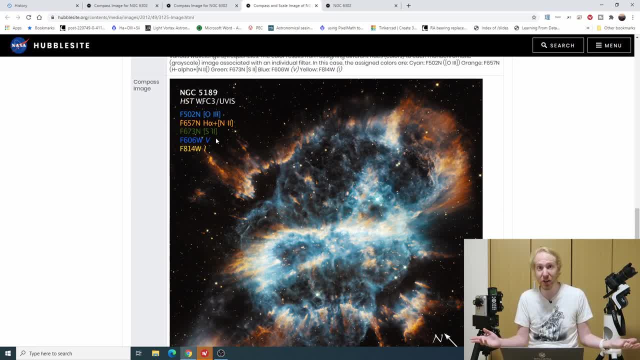 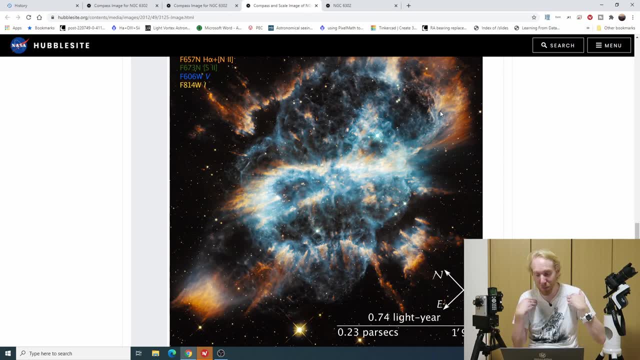 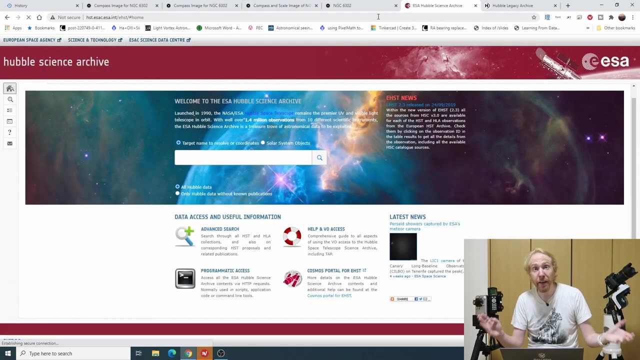 data, to do kind of feel like a standard Hubble combination of the data and see whether we can get something that looks like that, or whether we can get something you know that look better to me. And so to do so we'll have to go to the Hubble archive site and again I'll put the link in the 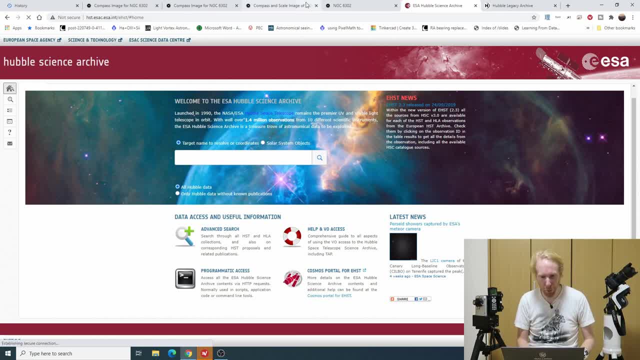 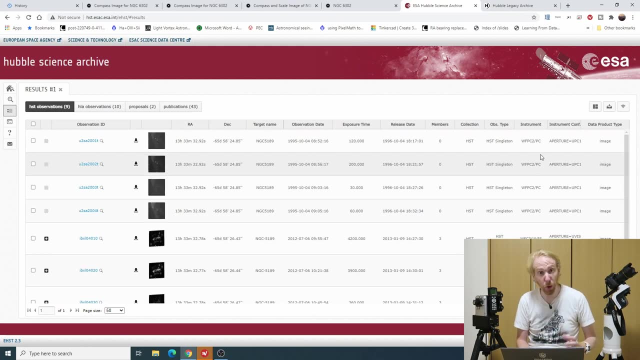 description down below. but here we are. we are on the archive and we want to search for ngc 5189, ngc 5189, and here it is. we're going to click search and we're going to get a lot of results in there. now, in the results that I get here, I want to add: 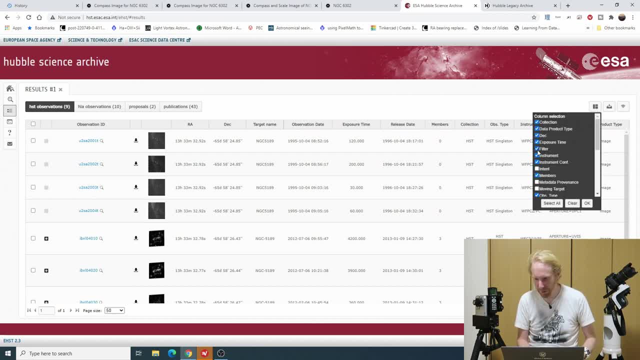 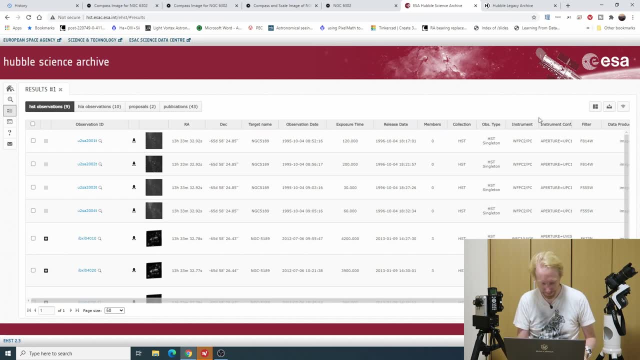 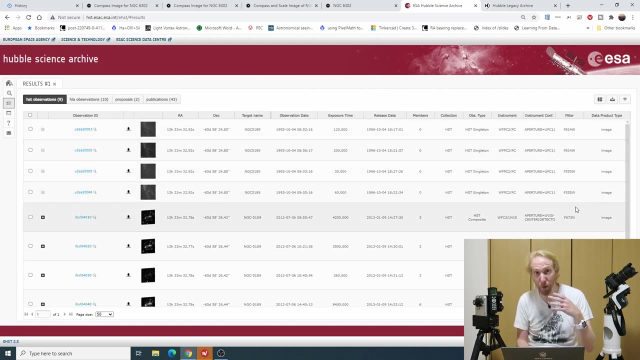 the filter column so I can click on this button, go to filter, say ok, and we should be getting an additional filter here. I'm going to zoom out a little bit. here we are and we have the actual name of the filter. and remember, we want 502, we want 657. 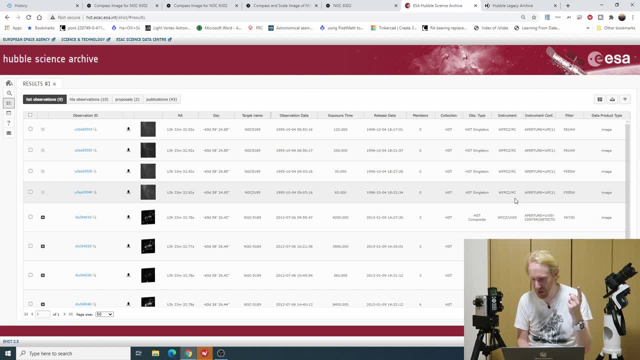 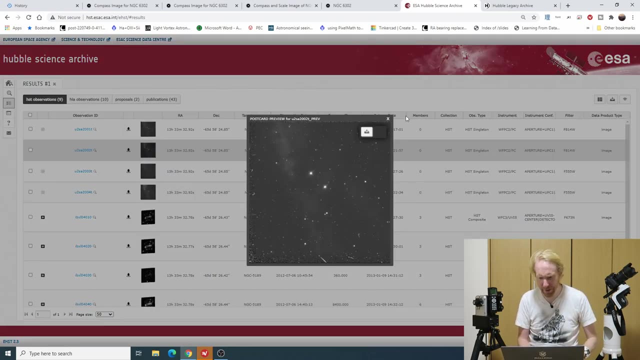 I think, or 656, and we have one 672. and one of the things as well that's very nice to know is that you have images that are like very single panes, and it's super interesting when you open them to see like all of those scratches that I see there, and I'm not sure exactly what they are, but they. 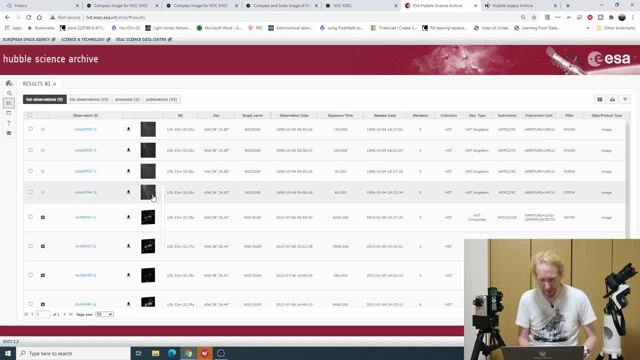 could actually be like cosmic rays or something like that. I have no idea, but a lot of those preview images have a lot of like small dots and and white dots and white lines on top of that that, and I assume that when they get stacked more they're able to be removed using pixel rejection. I have 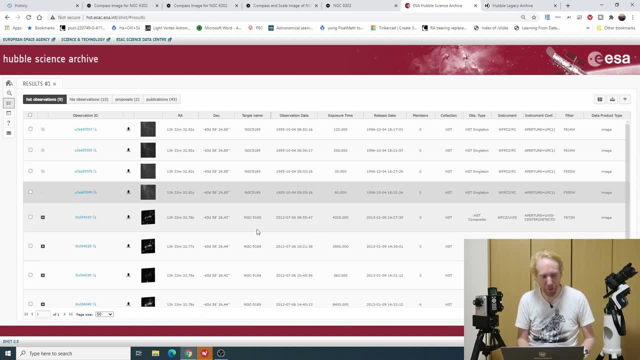 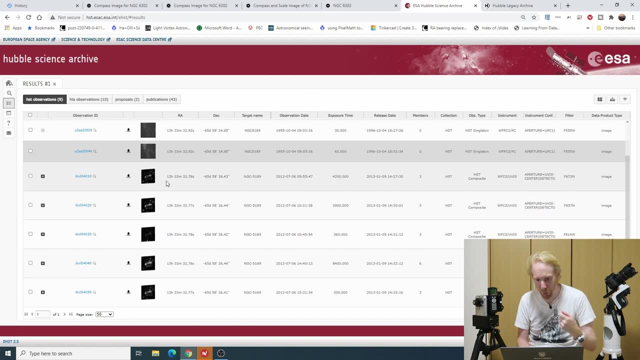 no idea how it works. it's a lot of fun to see that and some of the images they have a plus sign on the left hand side, which means that it's actually multiple images at once, and typically these are the ones that you want to re-look for, because they have, um, a wide field view kind of target, I think. 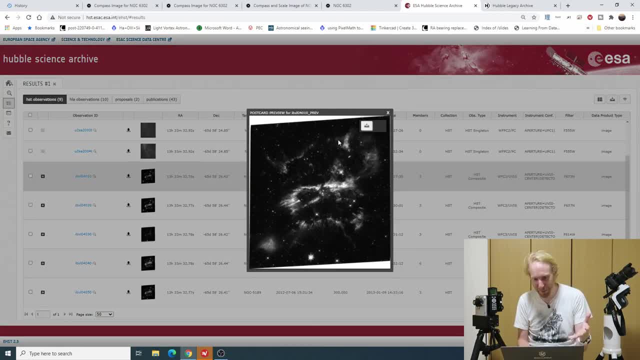 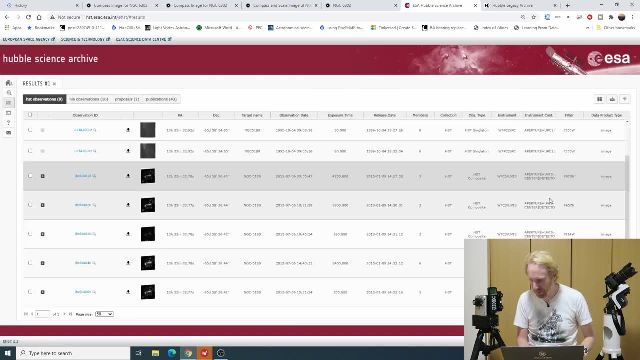 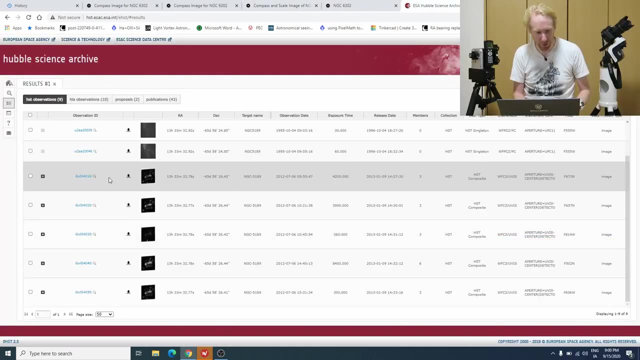 they're stitched and if I click on this preview. it took a bit of time, but here we are. we can see. this is one of the things that I want. this is exactly the object that I want to process and we can see it's 673, which means that it is indeed sulfur 2, so I want to download this and I'll just click. 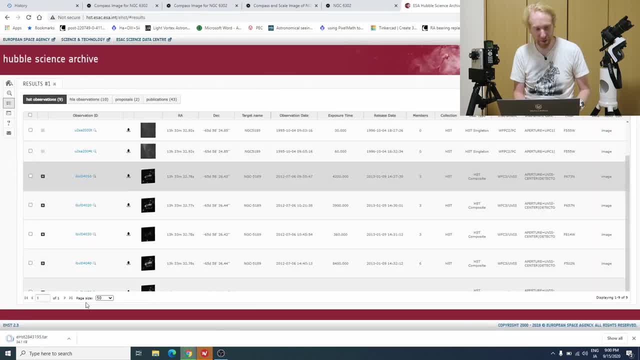 on that download button here and here it is, it's downloading, but it's like big, it's like 200 megs, something like that, per image, so it's not small. and then we have the next one is 657, which is h, alpha and n2. so I want to download that as well, and we want oxygen 3, which is this one, f502n. 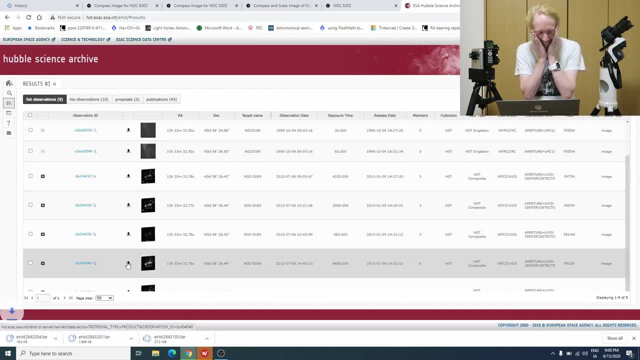 so I will be downloading that as well, isn't that? I love this. I'm downloading three images from a space telescope. they're raw images, they're fits files. there's all the data from that telescope. isn't it amazing? I don't know. I think it beats like any remote telescope in the world, like 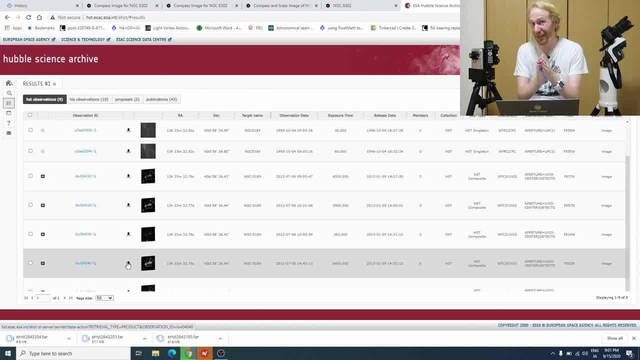 100 fold because I haven't. I want to try remote telescopes at some point, but I'm never sure you know how rewarding that will be. so it's like the Hubble is not rewarding because it didn't take the the images, but it's pretty cool. that is something that is in space that's still working right now. 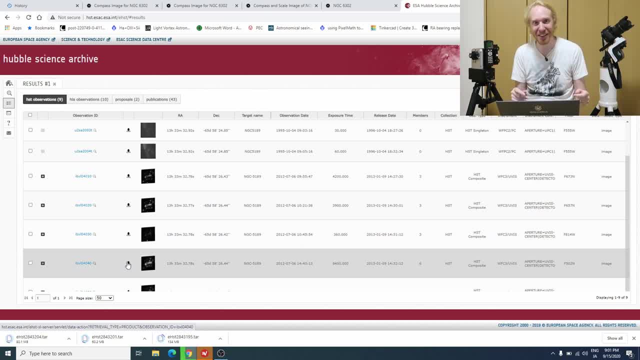 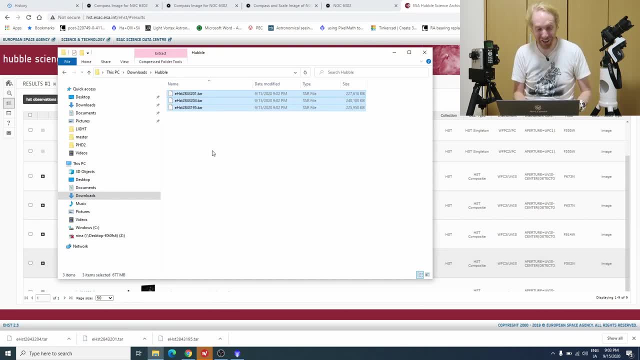 and, yeah, I want to see what that gives us, and so I'll be waiting for the download to finish and then we'll be opening that in PixInsight, okay, and the download is done. so I'm going to actually look at the files that we've downloaded. they're tar files and if you're running like Linux, 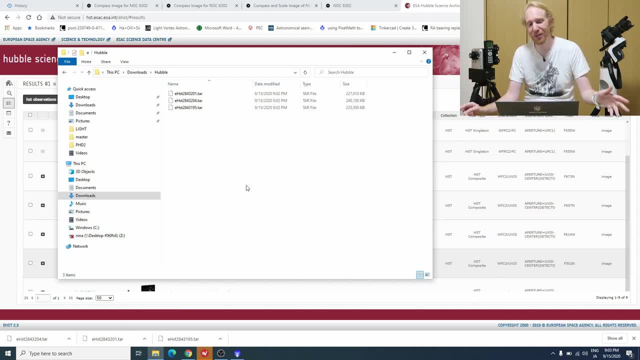 or macOS, you'll be have no problem opening those. if you're using windows, you probably want to have like a proper archive software like 7zip, which is what I use, and I'll be just right clicking on the archive using 7zip to extract to each of the respective folders. so now we've unzipped. 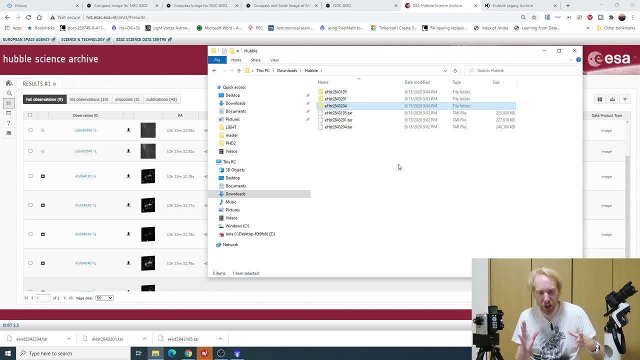 unzipped or unarchived them, and as soon as you extract the files, there will be a little bit of changes, and it's not quite clear which of those was H-alpha, S2, or Oxygen-3, right, So not to worry- in each of the folders. 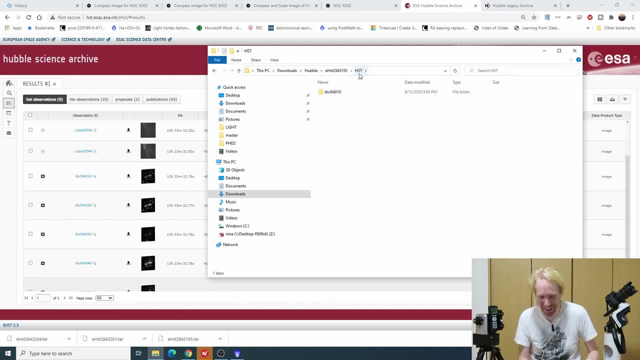 you'll have an HST for Hubble Space Telescope- How cool is that folder. And then you'll have the actual number there that corresponds to the ID that we have here. So we have 04010,, which means that 04010 is 673N. 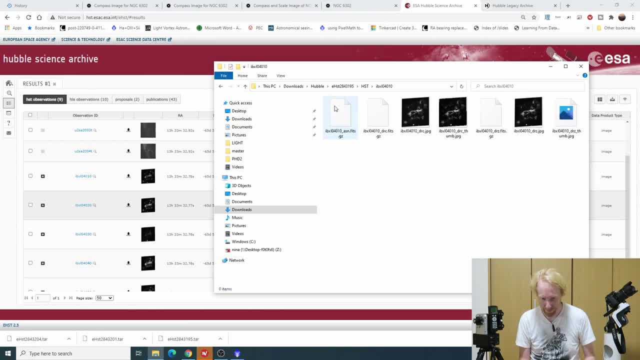 which is actually sulfur-2, as we saw. So I am going to. We have several FITS files in here, and one is 1.35 kilobytes- not enough. And then we have two that are each 109 megabytes. 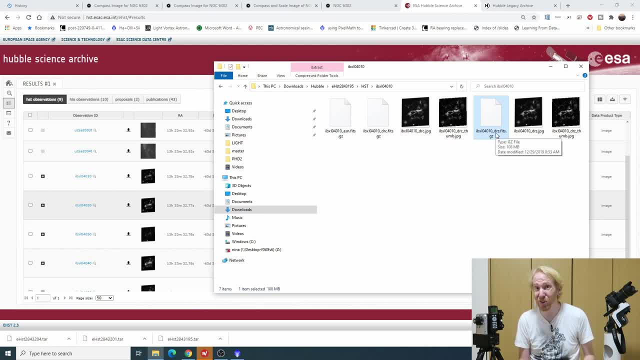 I'm not sure which is which, but this one has DRZ, which I assume stands for drizzle, And I like drizzled files. so I'm just going to use that And we are going to extract here, and that will extract a FITS file. 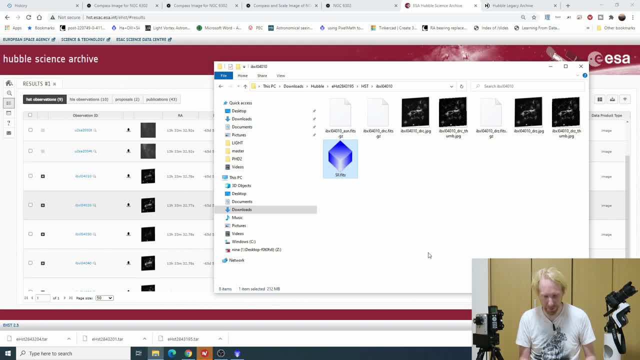 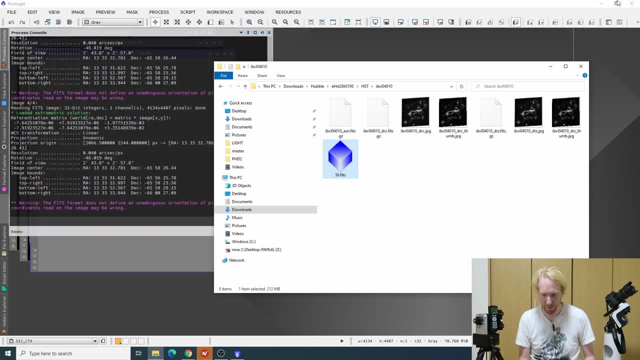 which I am going to rename to S2, so I don't forget, And I'm just going to open it in PixInsight while I'm at it. Okay, so the first one is opened. We have some rejection thingies going there. 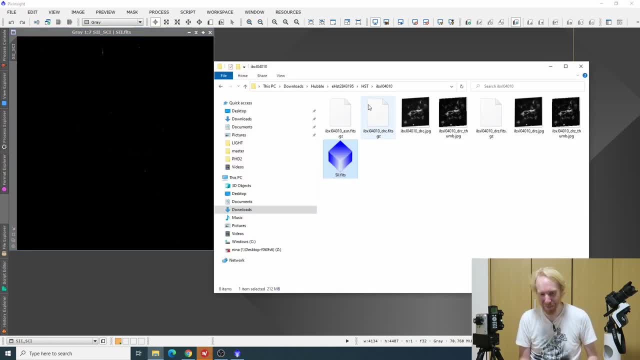 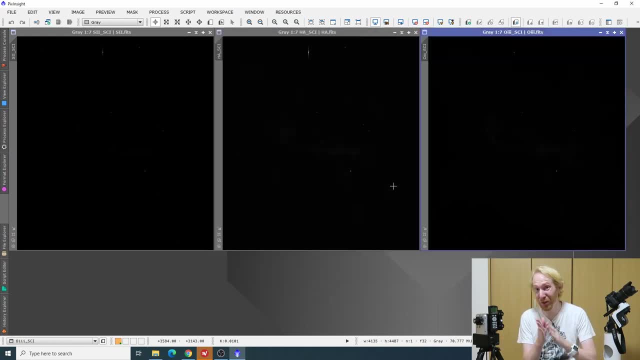 I'm not going to reveal the whole beauty of the image yet, And then we can go to the others and I'll do exactly the same thing. Okay, and I have all of my images open in PixInsight. Note that you'd be able to do pretty much everything. 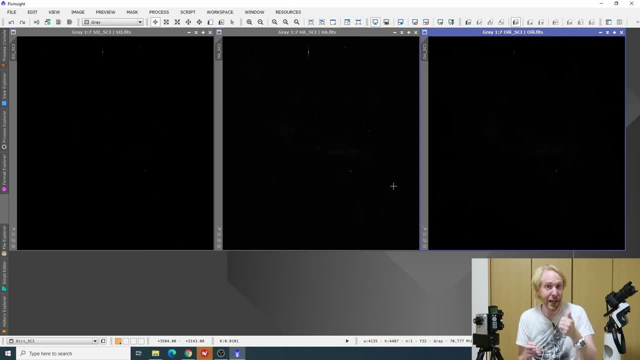 that I'm going to do to some extent using PixInsight. You can do layers in Photoshop or in GIMP or using the functions in CIRIL, free software that is available. Now I'm going to rename in PixInsight the various images. 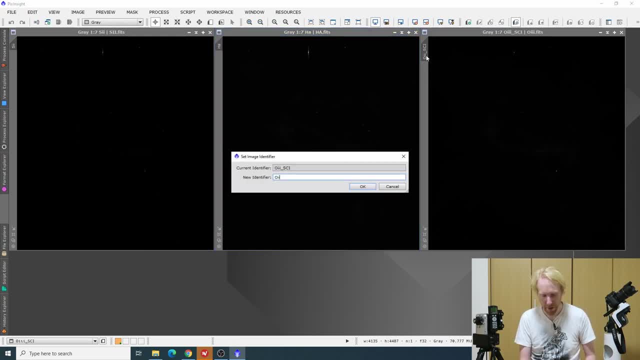 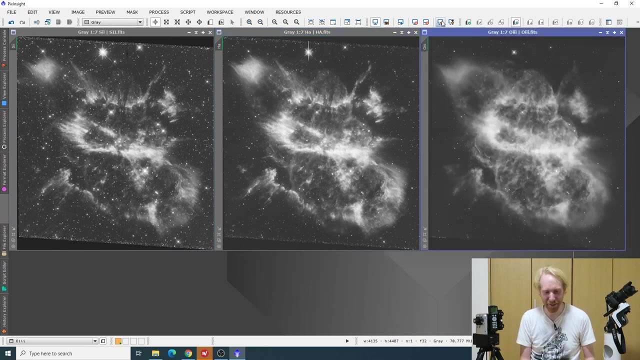 just to names that I'm used to using That way. I am sure that I don't have any problem when I do my combinations, And now we're going to look at it. preview how the data looks like. Yeah, I'd like to have this kind of data. 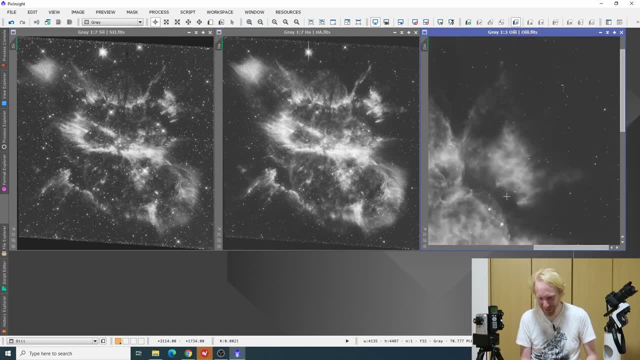 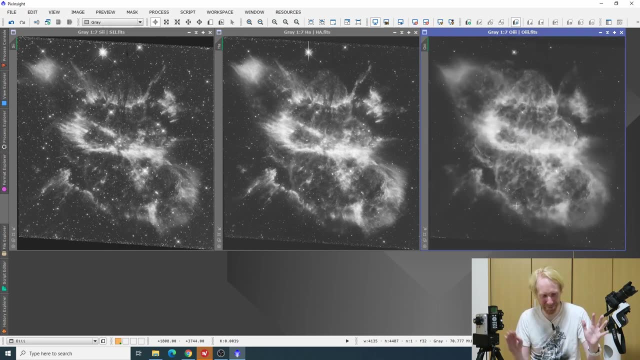 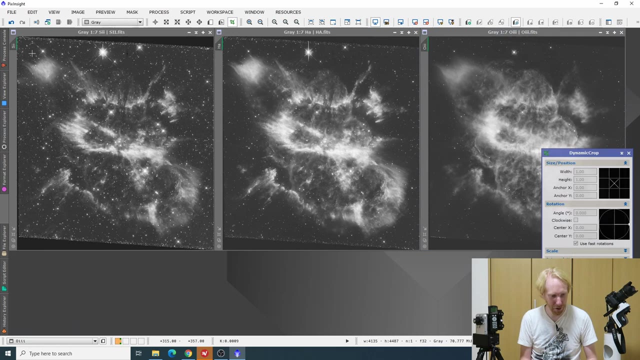 Look at Oxygen 3.. Oh my word, And this is so smooth. Oh my word, Ah, This, Ah, okay. Well, you know, enough admiring the beautiful data. I'm just going to crop that data using Dynamic Crop. 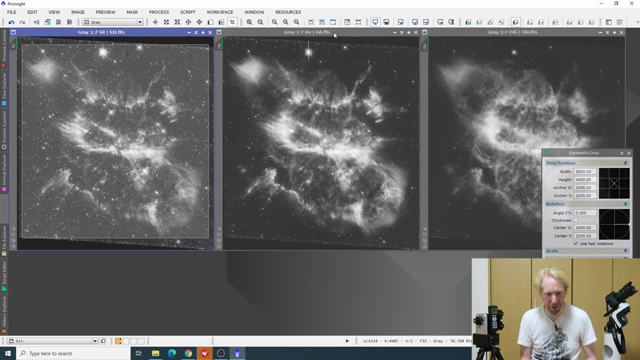 So I'm just going to quickly do something. Now. what's really cool is that those three images you can see they're already aligned, So they're really obviously part of a whole that already has been aligned, So it's much easier to process. 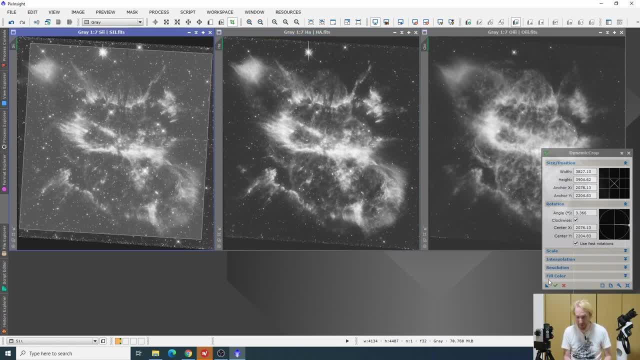 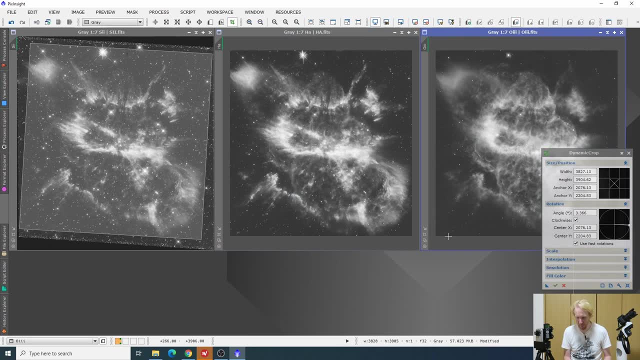 Okay, And I've made a crop that removes most of the stacking artifacts. I'm just going to apply that crop to each of the images in turn And, yes, I am okay with getting rid of my astrometric solution, which is embedded in that fits file. 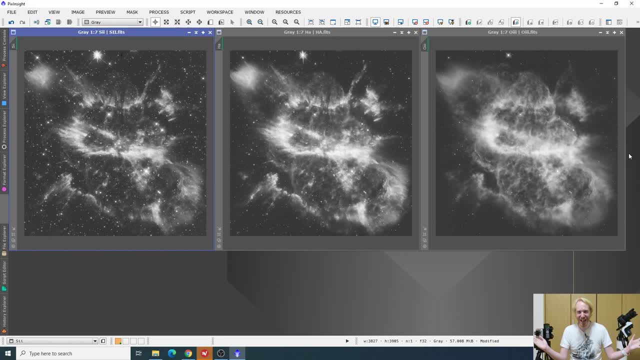 And here we are. We have the three images and I'm not going to. I mean, they're so freaking smooth. It's like- yeah, there's- ah, my word- like there's pretty much no point in doing like. 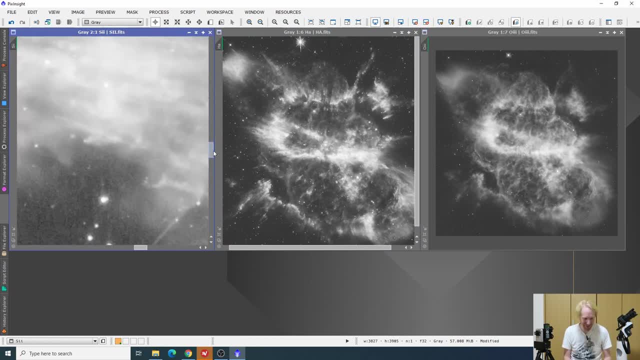 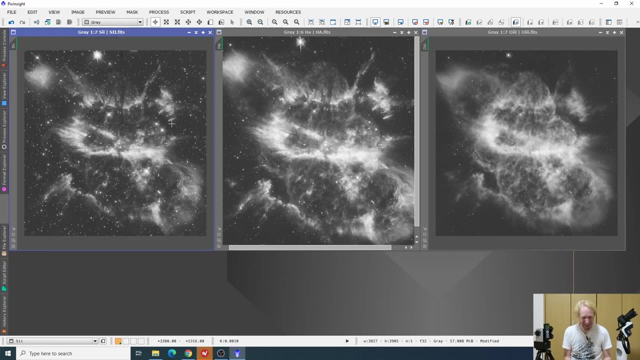 Oh, but this one has a bit of noise. S2 has a bit of noise. Even the Hubble telescope has noise. guys, It's shot noise but it's still noise. Oh my word, I'm not going to bother too much with like noise reduction or anything. 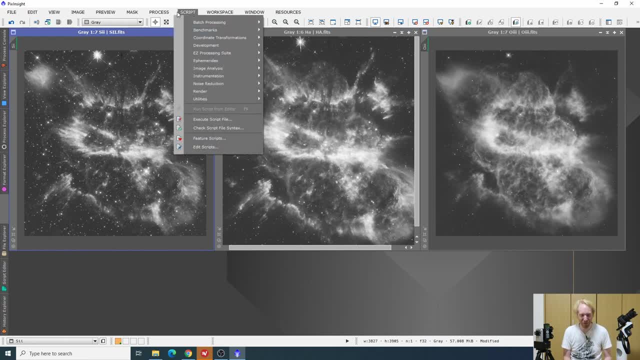 I'm not going to do any Anyway. I mean we want to do a quick fun processing of that And for that I'll just like stretch the images So I could be using. my usual preferred method is to use 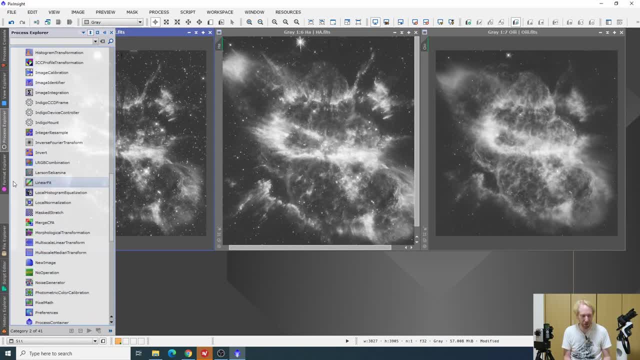 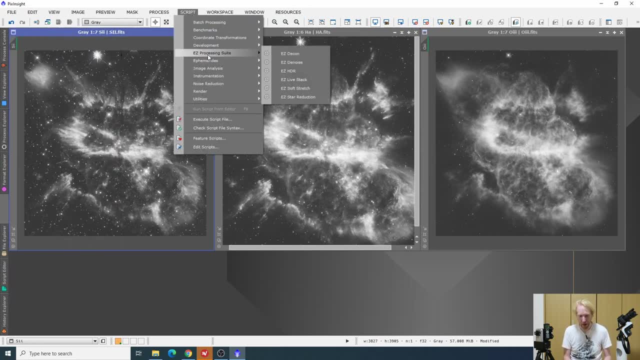 I'll use the mast stretch function in PixInsight. You can use a standard histogram stretch or you can use, like from the Easy Processing Suite, the Easy Soft Stretch, which I really like because it really brings the images to the same level. 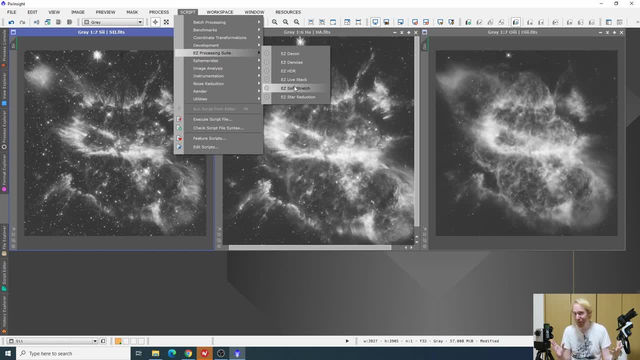 If you're not sure what Easy Soft Stretch is or what the Easy Processing Suite is, feel free to go and check up above. Or is it this here? I'll put a video about that. I have a video that I did in the past. 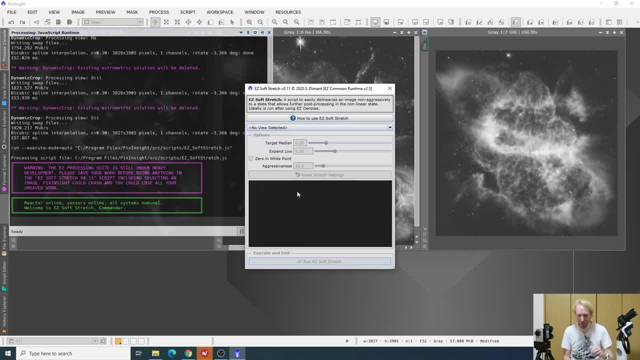 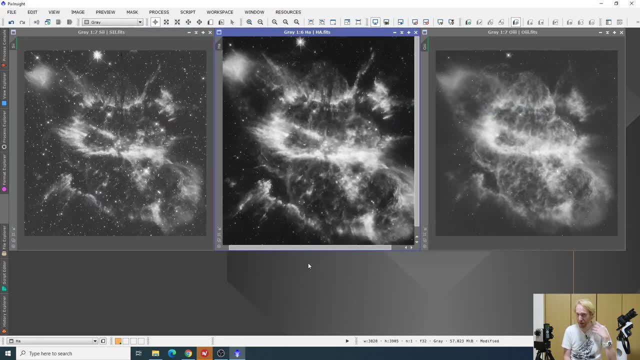 So let's apply the soft stretch to each of the images in turn. So I'll just select H-alpha. I'll just keep it as default. I run the Easy Soft Stretch and I'll do exactly the same on the two other pictures. 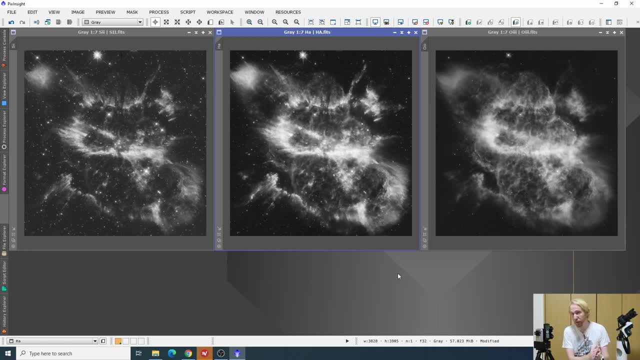 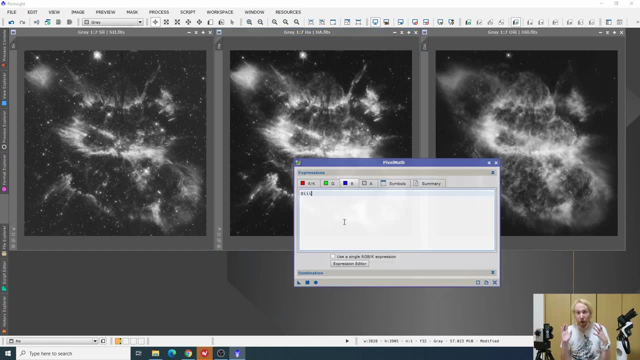 And here we are: We have three pictures that have been soft, stretched to pretty much the same level. So we are now able to actually combine them- And this is going to be the fun part- And to combine those images I'm going to use Pixel Math. 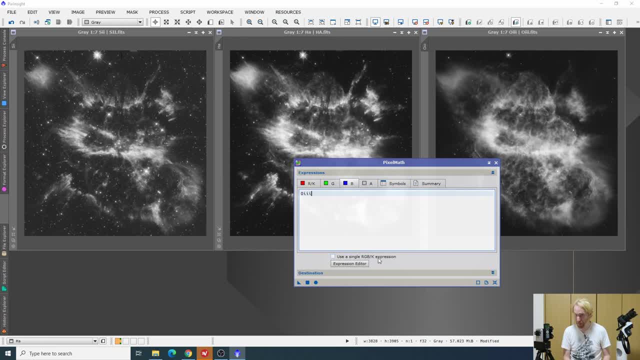 And I've unchecked the Use Single RGBK Expression because we want to use one color per channel, basically. But I'm not going to use a standard Hubble palette. I'm going to use 4-axis Hubble palette Or not Hubble palette, just 4-axis palette, which is supposed to be like. 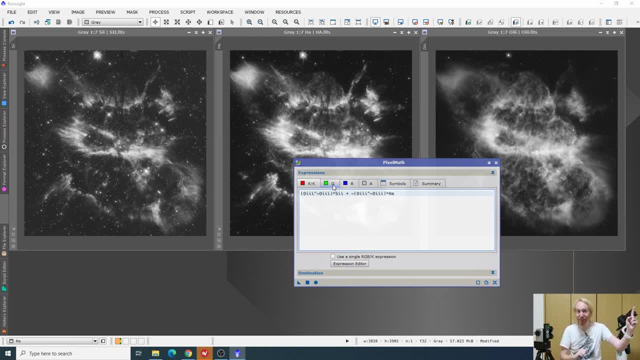 Which is really neat. I really like it. I have a video about that here that I'm linking to above. If you're also interested, I'll put a link to his blog post down below, because it is an amazing way Of combining that beta and we're going to see what that gives us. 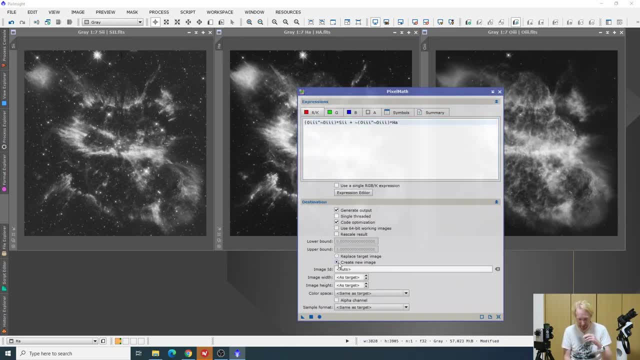 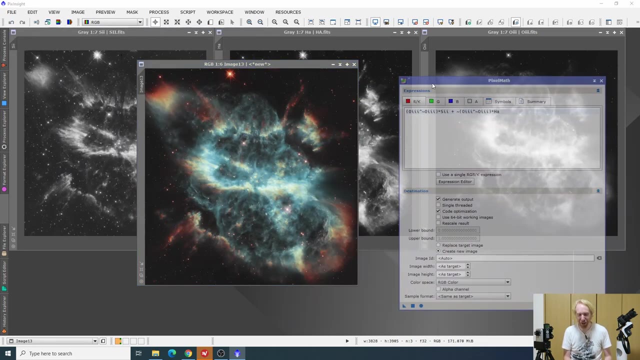 I want to make sure that in the destination of Pixel Math I have create a new image And I want the new image to be RGB color And then I'll press on Apply and that should create a new image. It already looks really neat with the colors. 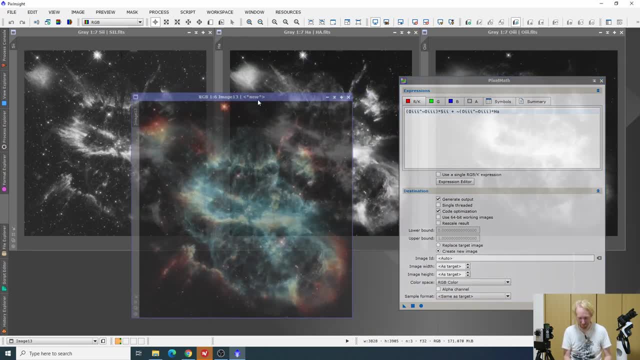 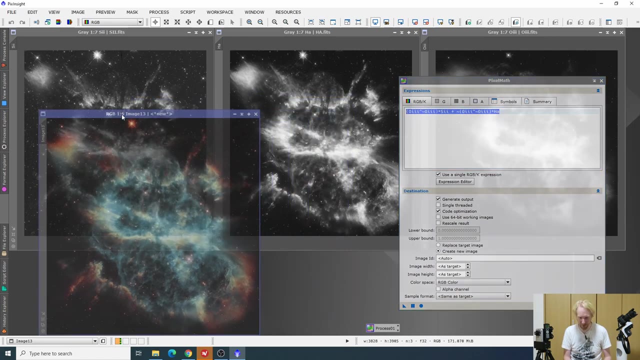 At the same time, I think I'll create a luminance image. And so to create a luminance image, I'm just going to save that process. But to create a luminance image, I'm just going to see that most of the signal is H-alpha and oxygen 3 with a bit of sulfur, 2.. 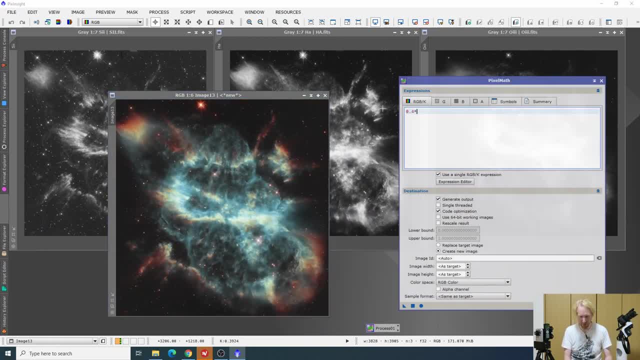 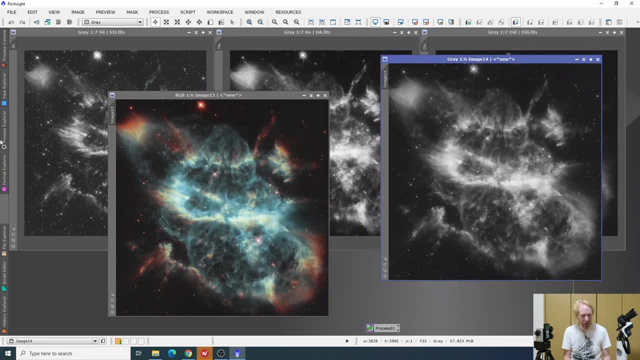 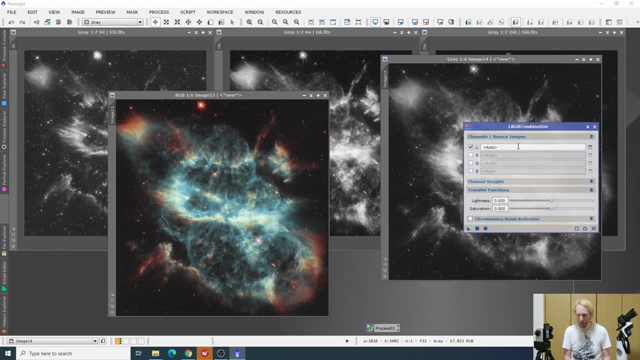 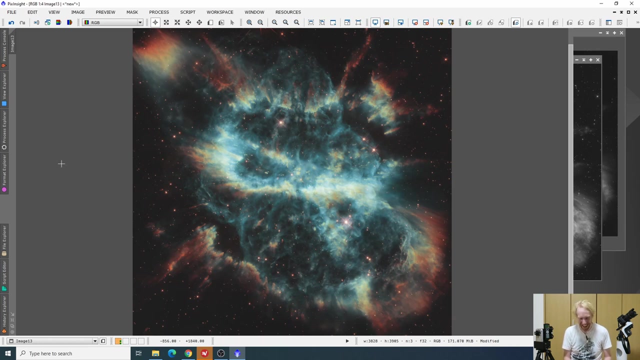 Now we have a proper luminance channel And we're going to use that luminance channel to apply, using I just created from the individual images, to our image here. And here we are. This image is already- And wichtig to our message- really cool and we can play with the colors, we can play with the hue. so I can 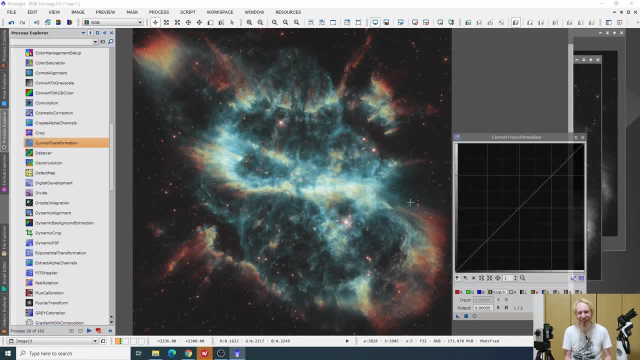 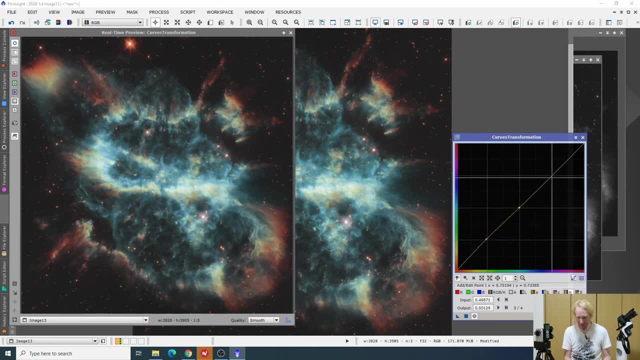 try to go, you know, inside the curves. but oh my word, this is so much fun. you know, playing with such beautiful data is absolutely amazing, so I can use like a hue curve to see, like how things you know change by moving things around. but maybe I don't really like hue curves actually, so I might just do some SCNR. 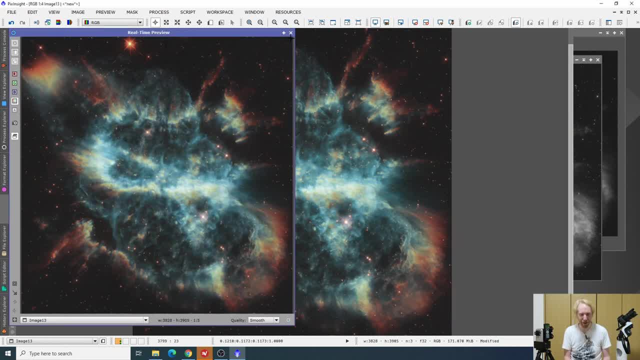 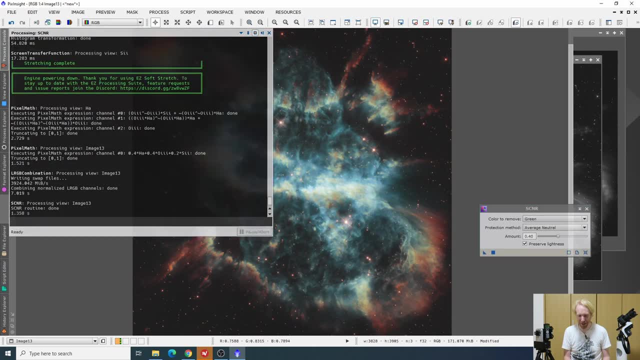 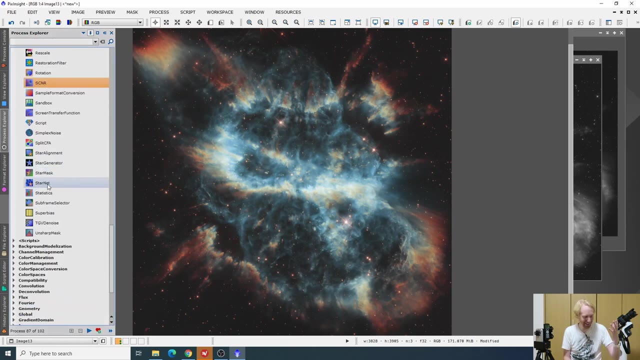 but this is so much fun. so let's actually do some SCNR to remove a bit of the green whilst while keeping some. so I'll put the a fairly non-aggressive setting at 40%, and here we are: we have a bluer color, and I can just like it's so. 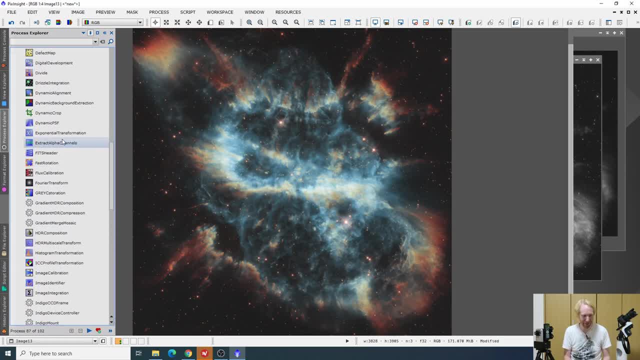 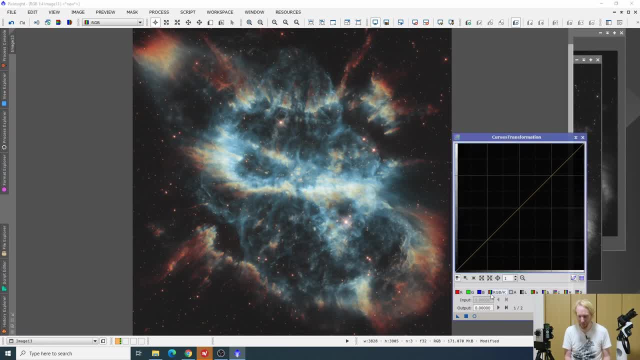 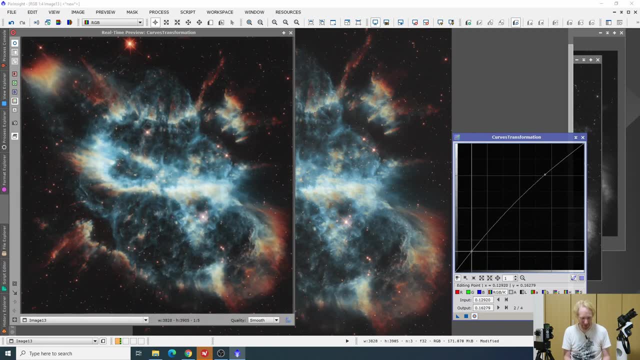 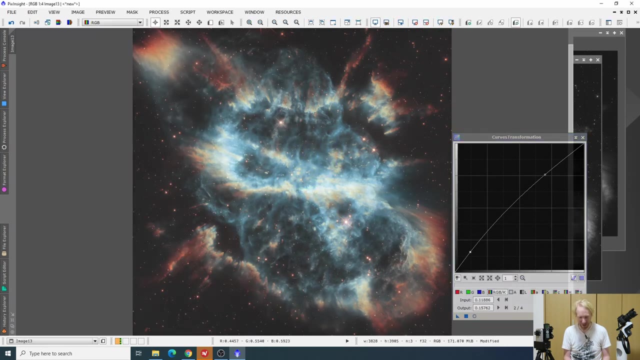 for anyone who is, like, responsible for bringing, like the Hubble data to life. because it's just like, it's too easy. I can do a small like curve to get out more luminosity, more nebulosity out of this, out of this image. I can just like. 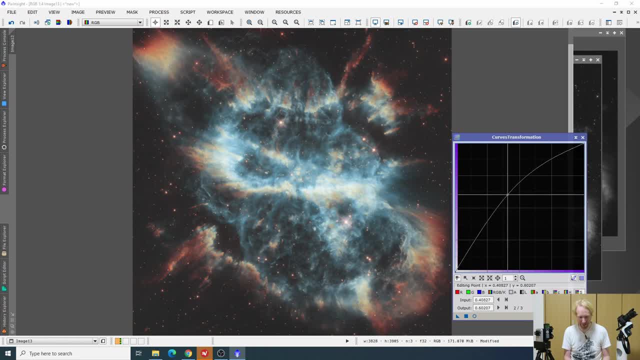 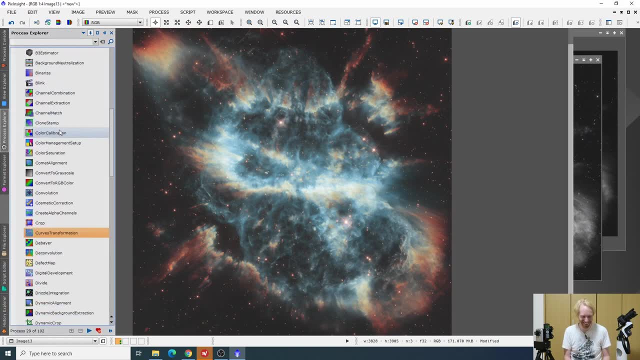 go ham and just like saturate the image a bit, or maybe we're gonna saturate the blue a bit more than the rest. it's like wow, the sky is the limit. so I can use a color saturation curve like that to specify like I want some. 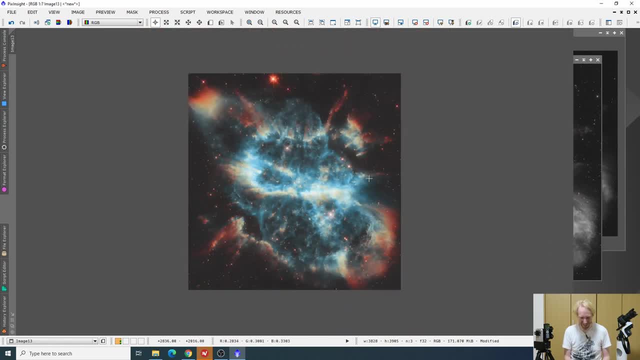 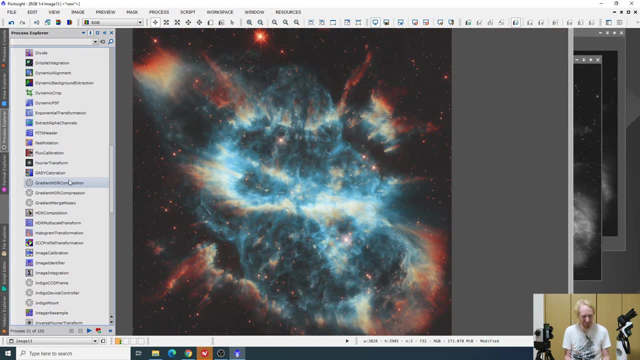 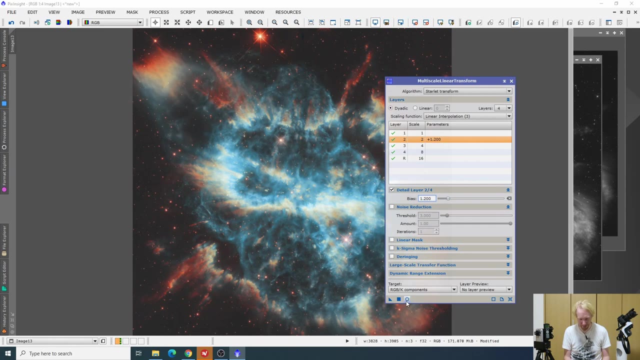 more colors there and man, how amazing is this. and the details in the image. I think we could do deconvolution, we could do some. I'm gonna do some simple sharpening, I think, like multi-scale linear transform, maybe a little bit at a scale of of two, something like that is pretty neat. we could do some local. 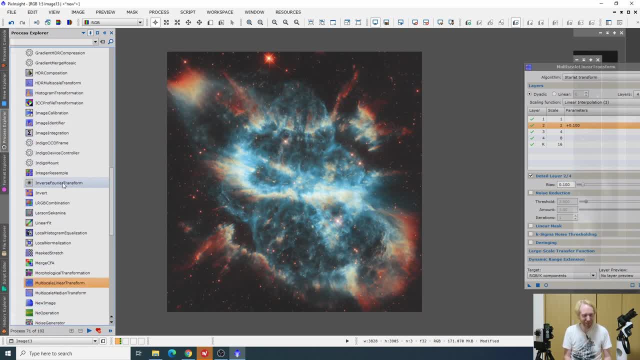 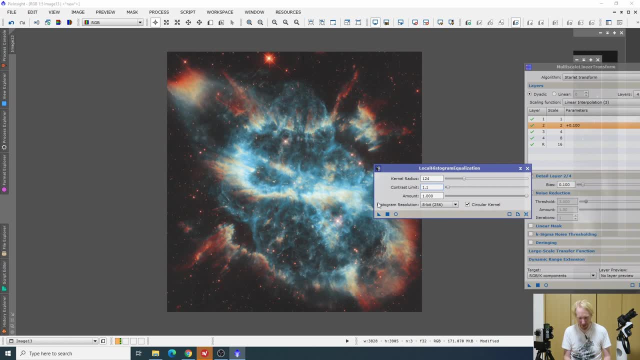 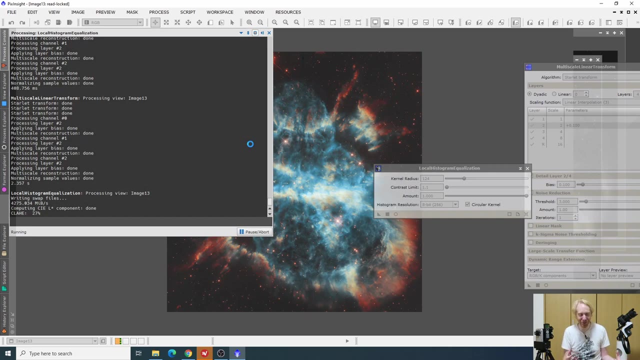 histogram equalization. you know it's like it's so much things that you can play with in this image that it just blows my mind. I can be very conservative on the local histogram equalization. there's almost nothing to do and I really like the color scheme that we are getting here. we 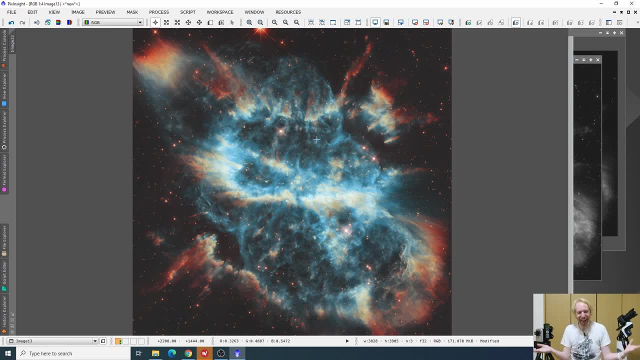 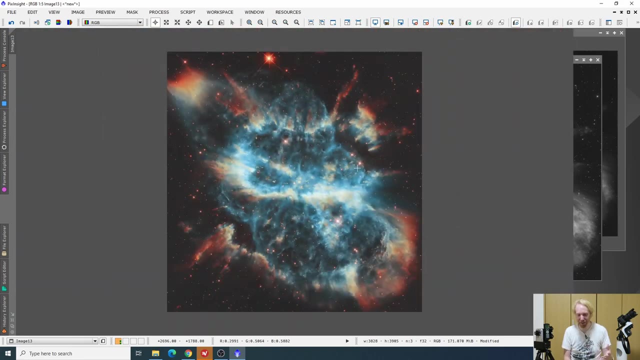 are. I think we're getting a decent result here already, like we didn't have to do anything really, and this is so amazing. it's a lot of fun because with such clean data, you can really test a variety of like processing tools without having to worry too much about noise or things. 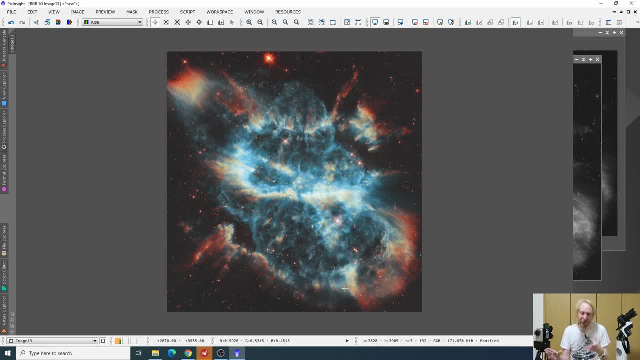 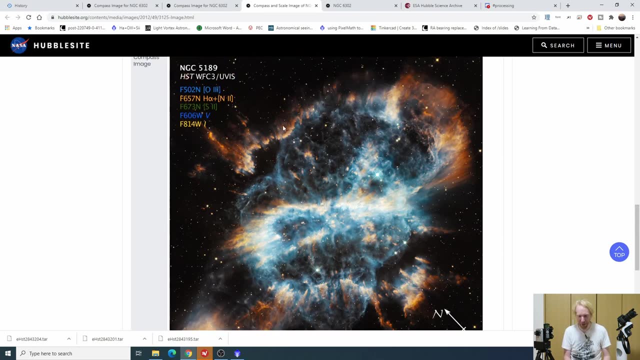 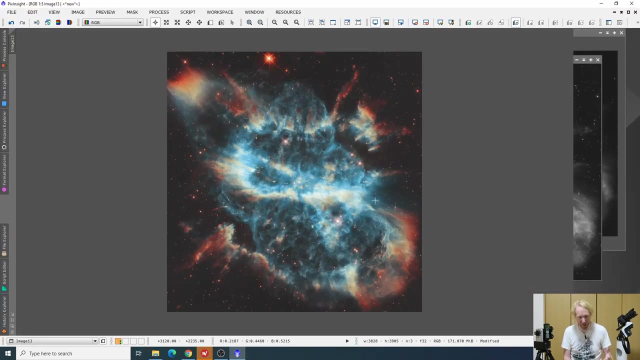 like that you can try to extract the stars and, you know, play with the nebulosity itself and I find it is so much fun and I, you know, like, compared to the standard, like Hubble palette type of colors that we get here, which is very much by color, the, the tricolor image, a proper tricolor image that I get from. 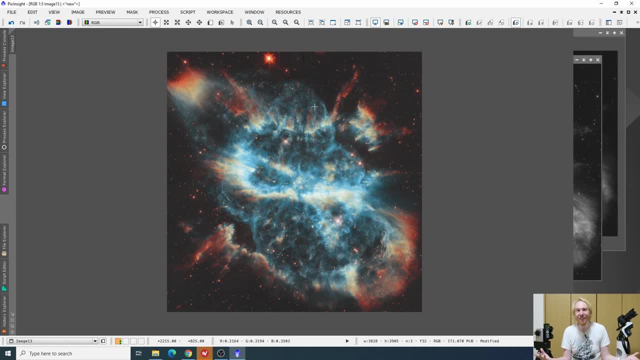 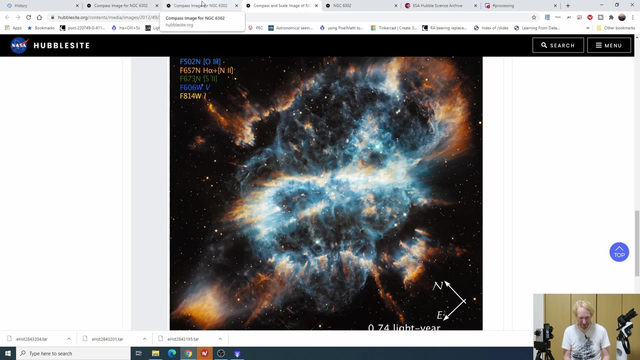 here. I kind of prefer it. and then there's tons of everyone can have their own little variation of that and I find this absolutely awesome. so I'll be, just for the fun, processing another image. so that's one of the images that I saw on the very first page of the Hubble images site, which is this one, NGC 6302. I'm 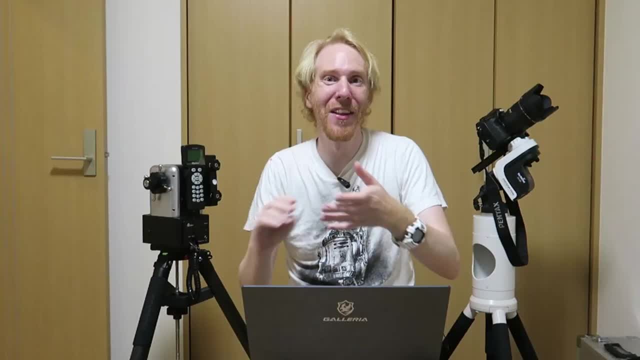 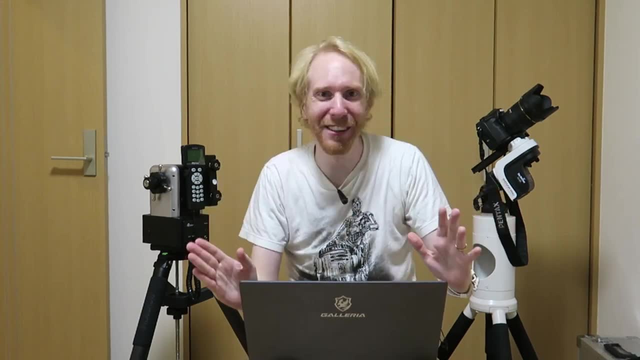 gonna put that, along with that first image, at the end of the video. oh, and that's pretty much it for this topic. I think I hope this was. this is a good idea. this is something you'll want to do. I'm personally loving this. I'm going to. 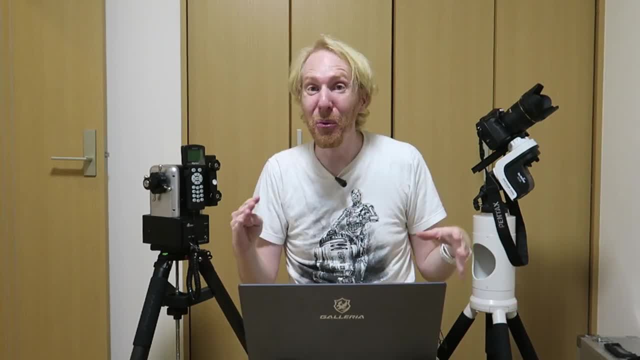 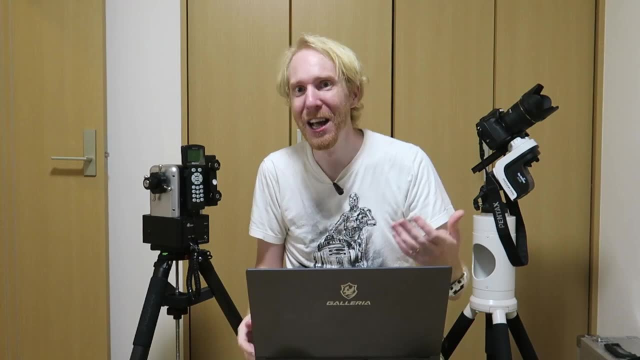 spend hours on this. this is just so much fun and I hope you enjoyed this video. it's too much fun, so with that, thank you so much for watching. if you're not a subscriber first, welcome to the channel. this is a channel mostly about astronomy, astrophotography- I am Quiv, based in Japan- and tons of videos on the.